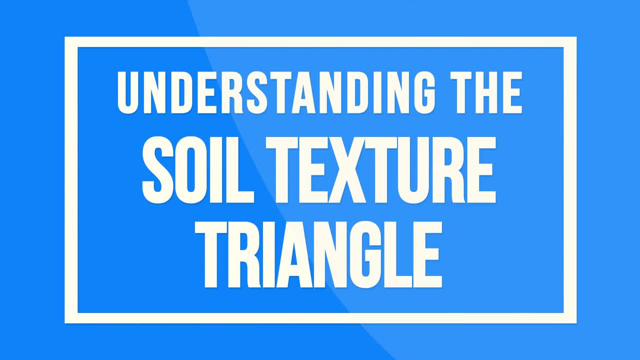 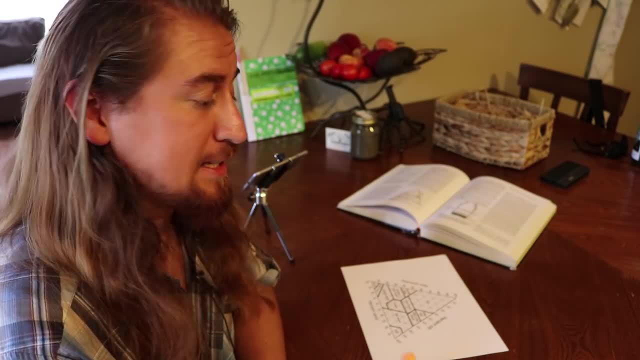 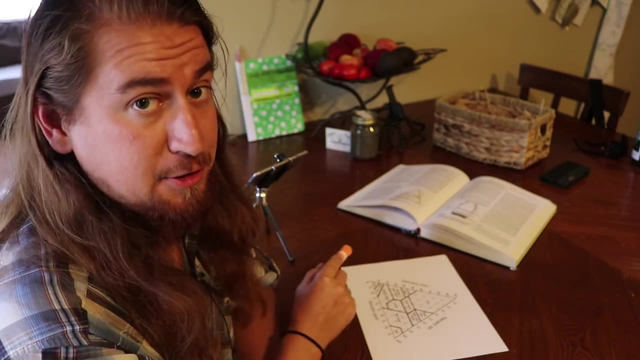 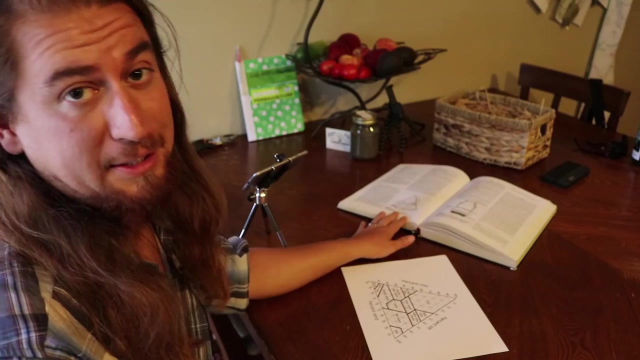 Guys, you take a permaculture design course, you go through the soils class, you learn a ridiculous amount of information, you do your own study and you get back to Permaculture Designer's Manual Flipping through here page 186, you have this amazing, super complicated. 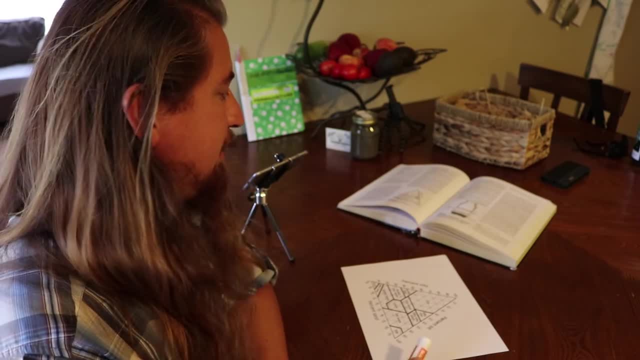 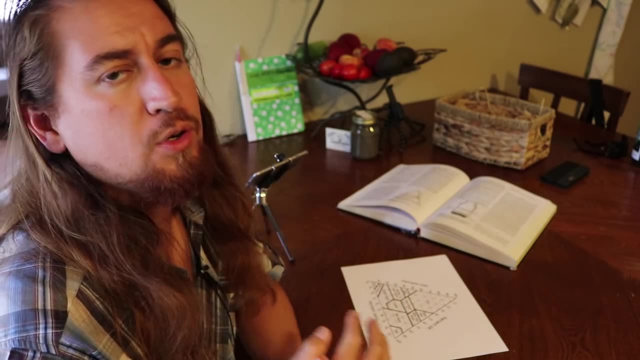 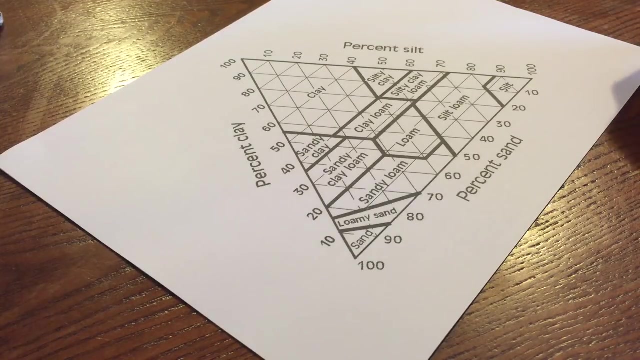 looking graph. What is that? That is the USDA's Soil Texture Triangle. So what in the world is a Soil Texture Triangle? Well, it is not a triangle to be concerned about. It's pretty simple to understand and the reason it is there is. so we can take something simple like: 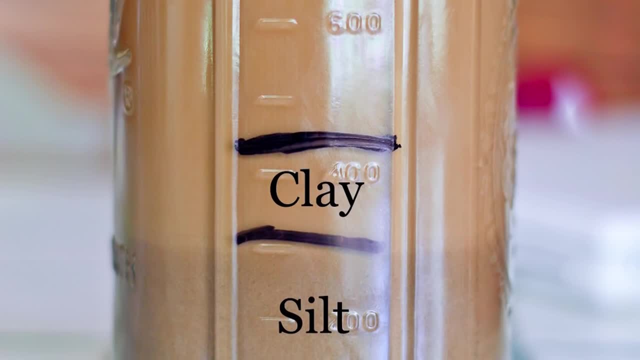 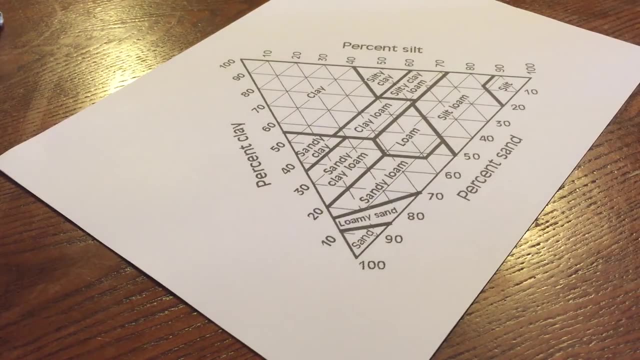 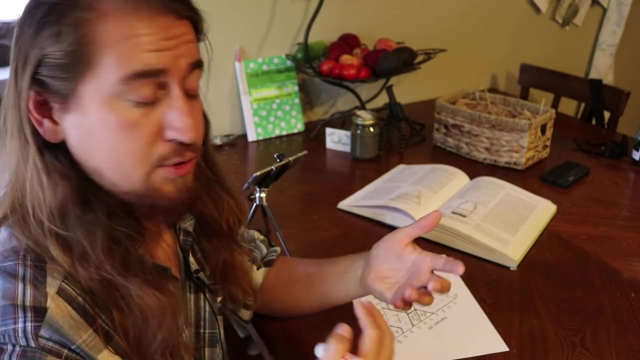 that mason jar test that we're always doing. we can use that, get our percentages of sand, silt and clay And we use those percentages to then properly identify them into a category that the USDA will classify and recognize. Then we can use that wording of the classification to further. 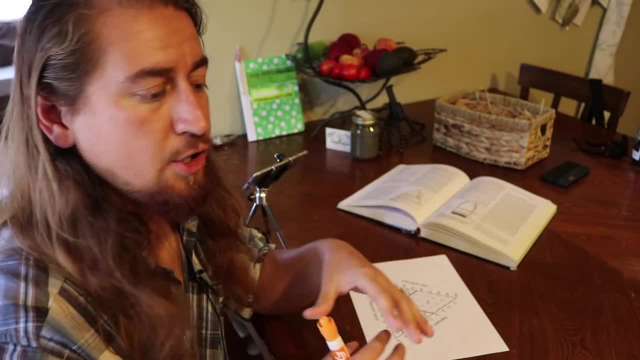 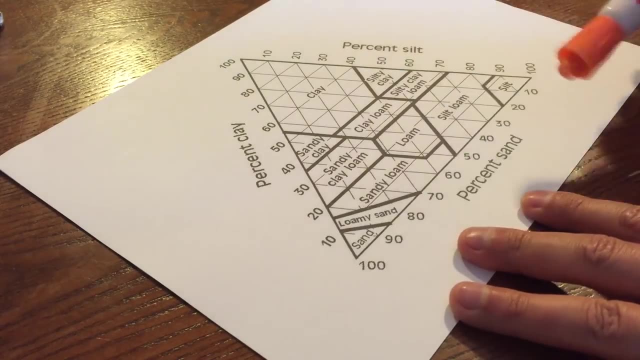 like: maybe go on to talk to geo-environmental engineers or whatnot if you're wanting to build a pond or a dam, So let's go over it. Okay, looks very complicated, but in actuality it's really simple. They've already put down. 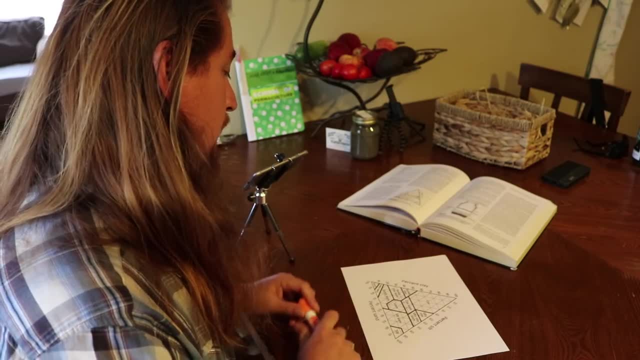 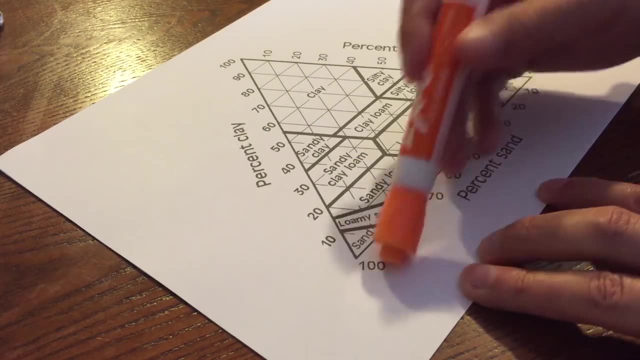 the blueprint for it. You just have to fill in what is what. So let's look at this: This side of the triangle is clay and this side is silt and this side is sand. And, if you notice, we start here. it starts at 10, up to 100, and then 10, down. 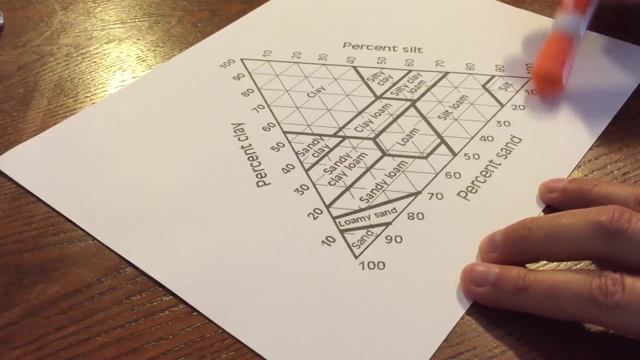 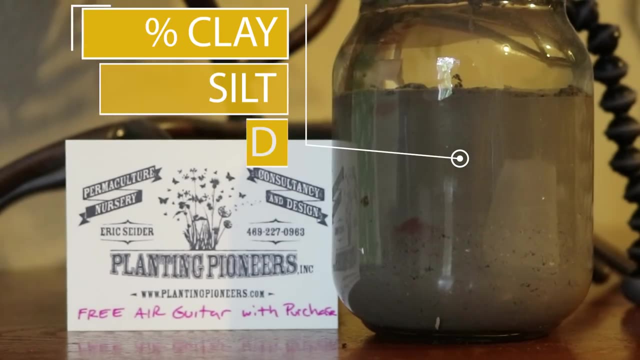 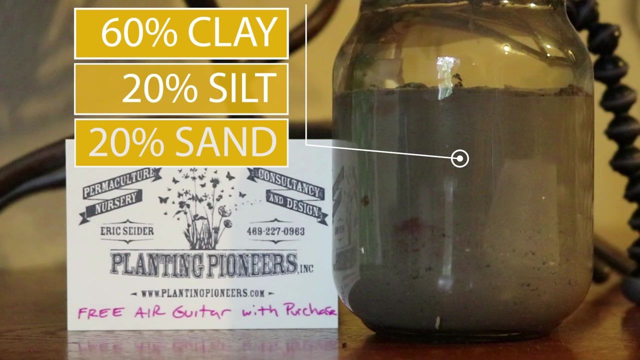 to 100, and then 10, across to 100. So it's kind of this like triangle-y circle. Let's look at this soil type. If we get close up on it we can see that it's about 60% clay there at the top, And then underneath that you'll see an additional. 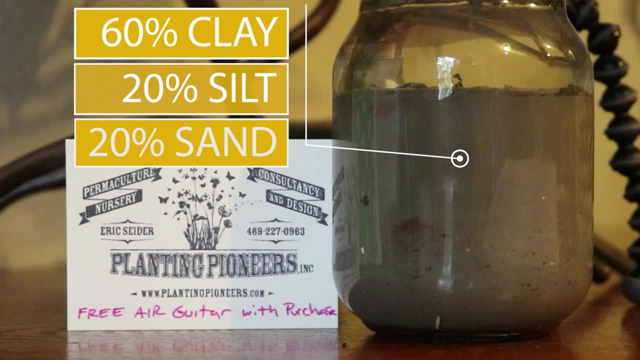 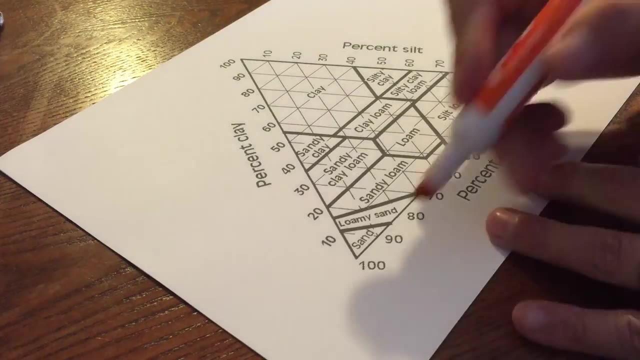 20% of silt and below that it's 20% of sand. It's very difficult to see, but you can see the structure changing as you get close to it, and they're all very similar color. So how do we reflect those numbers onto this chart? Okay, clay side, We're at 60%, so 60%. 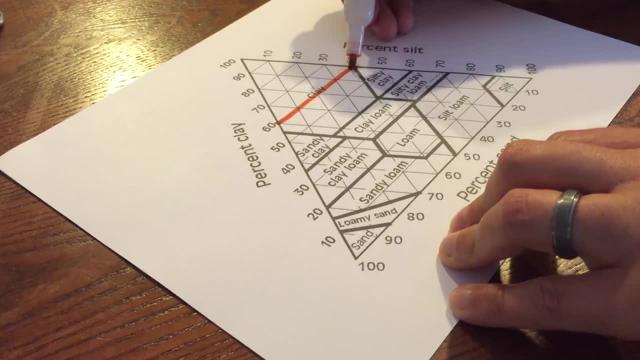 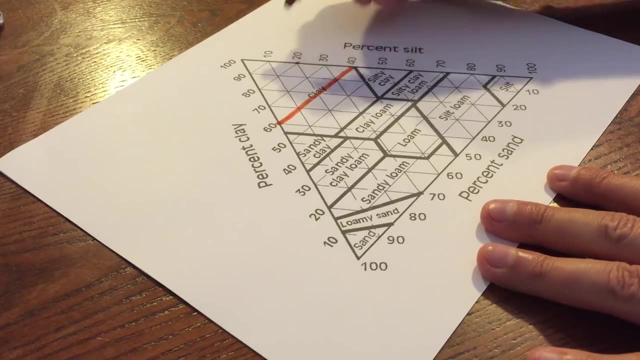 is right here. We're going to move horizontally. We're going to move horizontal like this. So the clay is on this side and it moves horizontal On the silt side. we're at 20%, so it starts here. This one goes down on a diagonal path. 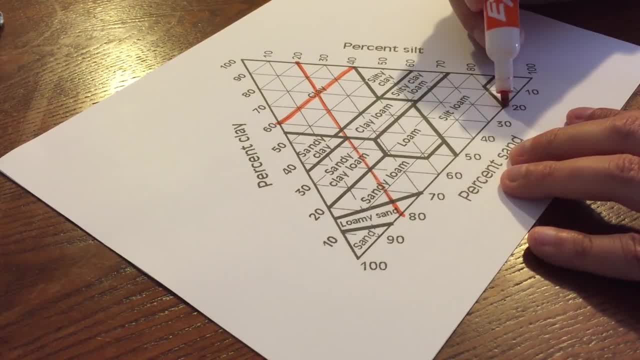 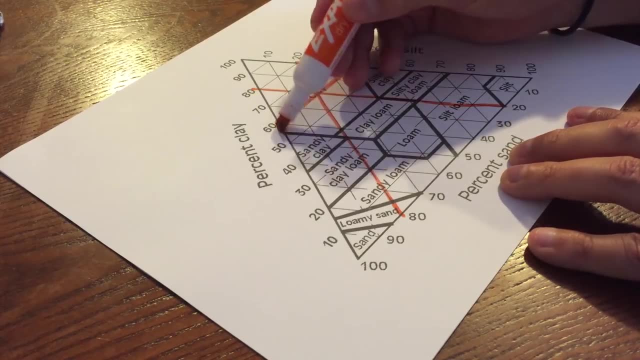 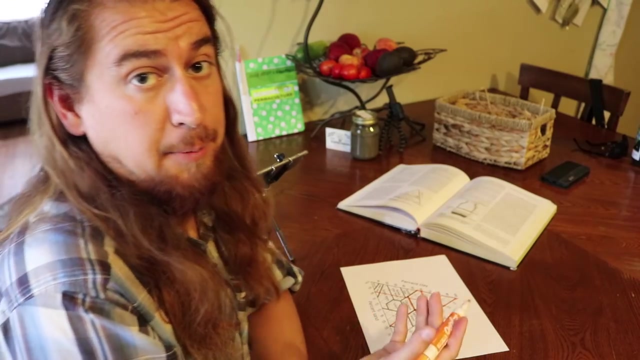 like that On the sand side. we're also at 20% and this one goes up. So where these intersect, boom, It's in this whole piece of the graph here. that's clay. So we can safely say that the soil type in this mason jar test that we have done ends up being a clay soil. 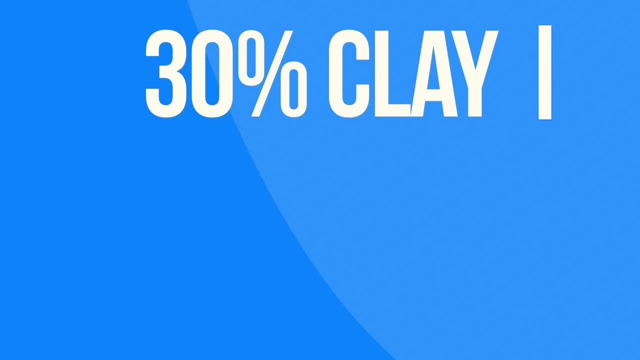 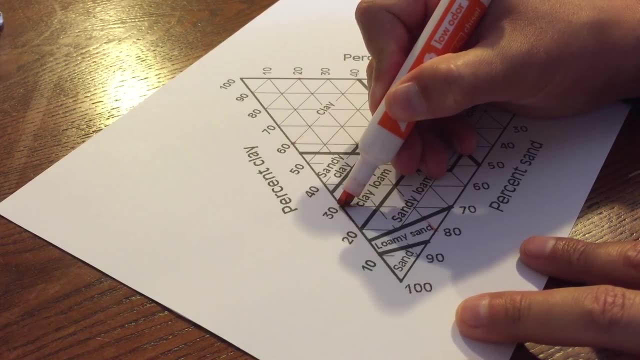 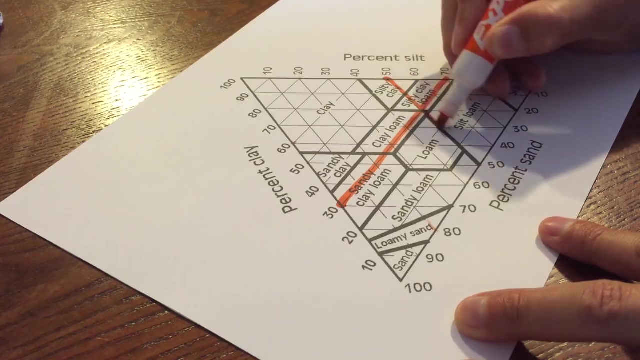 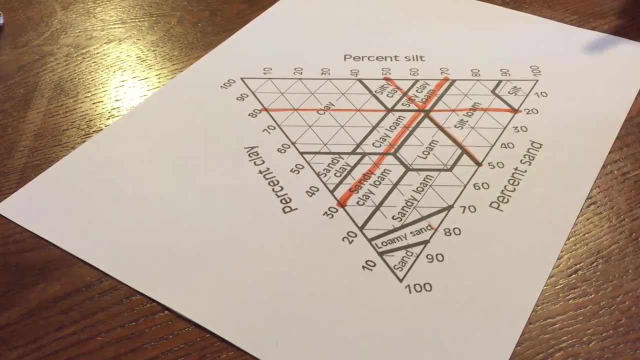 Let's do one more. This one is about 30% clay, 50% silt and 20% sand. So here we are, We're at the 30% clay and we'll come across like this: The 50% silt down and the 20% sand. Boom, Right here. 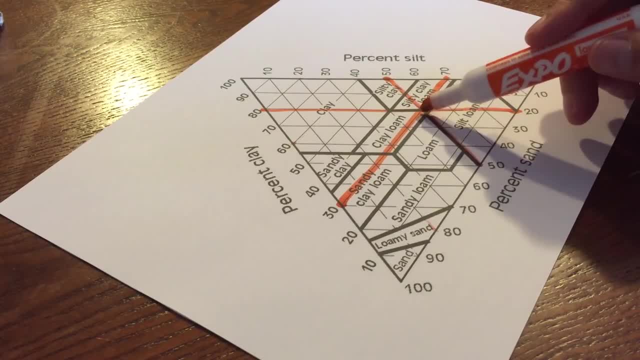 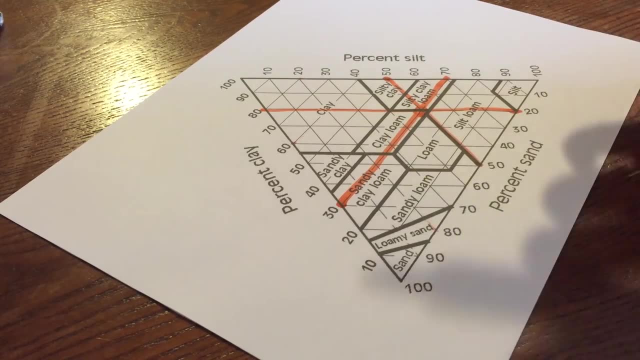 This one is right in between the silty clay loam and the clay loam, Like right in between, right there. So that has almost a dual classification, but you can classify it now in one of the categories with the USDA's Soil Texture Triangle. You guys are awesome. Make sure to check out. 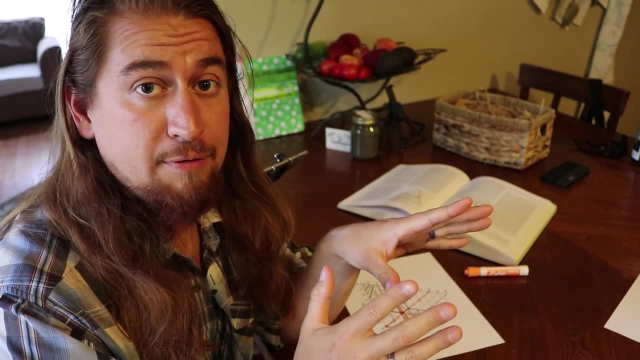 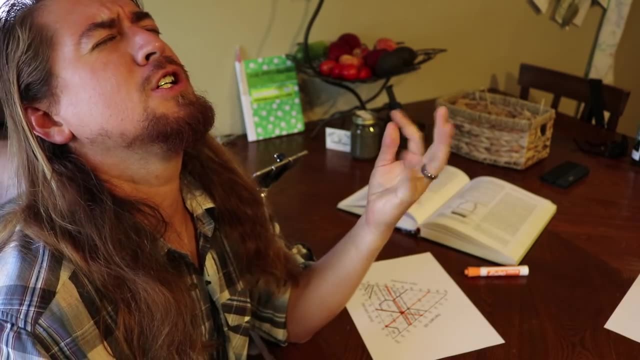 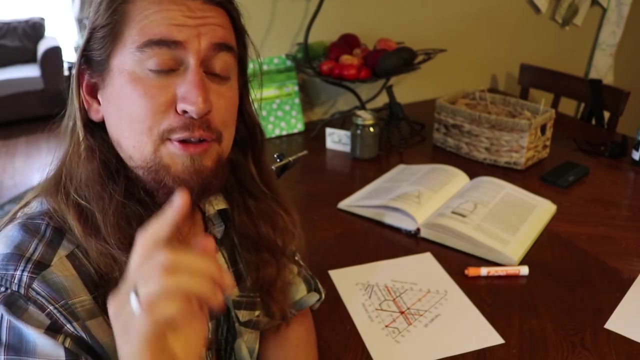 schoolofpermaculturecom. Check out our Facebook page, Come and like us, Subscribe to our YouTube channel And, by the way, right now, just play some air guitar. You get a free one every time you come to class. It's amazing. I got a whole house full of them. Know that. the proceeds from 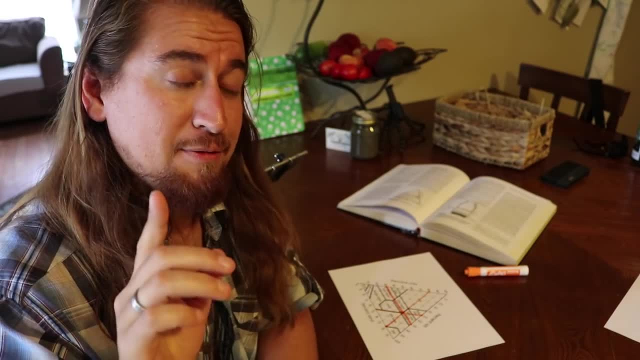 both of those go to our aid and our orphanage work and where we invite you to come and learn more about soil texture. So if you're interested in learning more about soil texture, come out with us and hang out and just love on people and help them using the tools of permaculture.